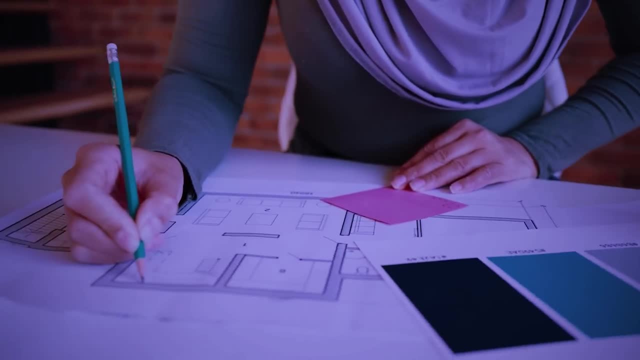 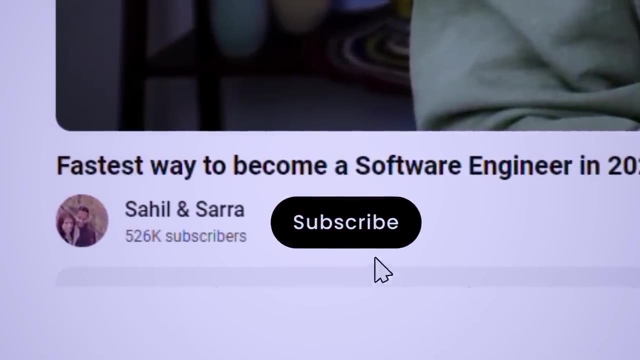 be a like and subscribe button here. CSS is like an interior designer that decides what your rooms look like For YouTube. it decides the shape, color and size of the subscribe and like button. When you hit the subscribe button, the color of the button changes. That's also CSS doing its. 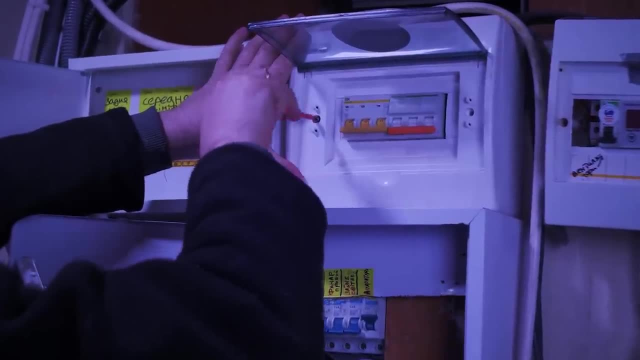 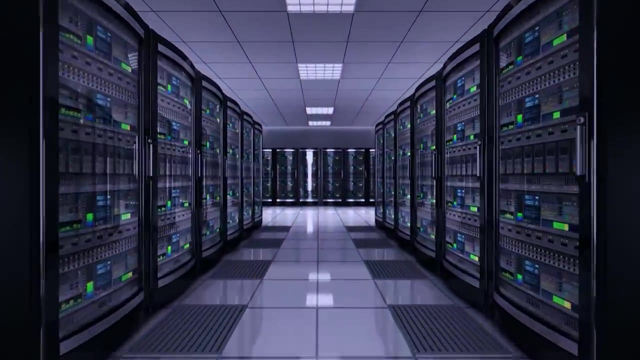 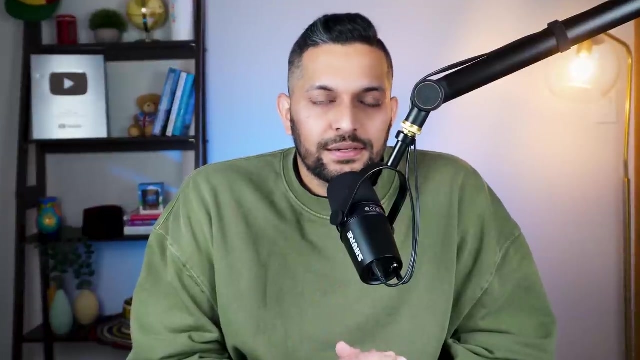 magic. JavaScript is like an electrician that installs smart home features in your house. In the YouTube example, when you hit the subscribe button, JavaScript sends a request to YouTube servers to update the subscriptions of my channel. YouTube servers will store this information and use it to recommend my next videos to you. Now that you understand the basics. 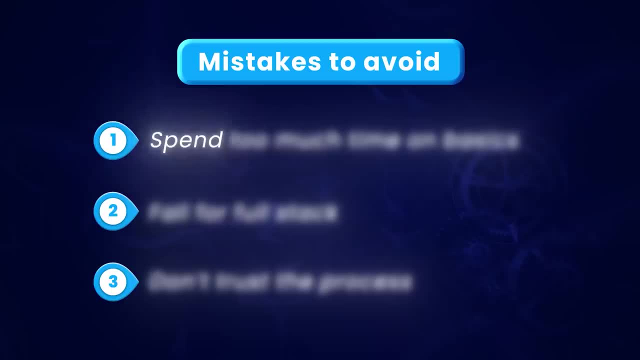 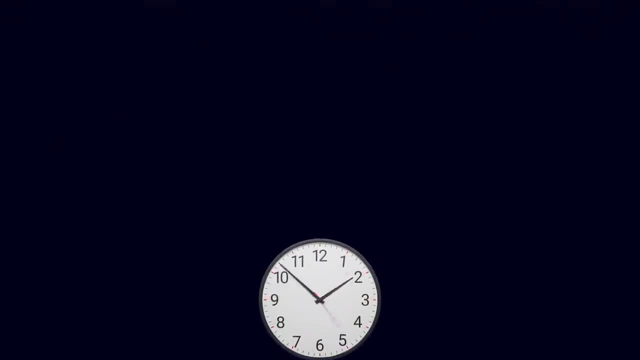 let's see how we can learn HTML, CSS and JavaScript, And this is where most people make their first big mistake. They spend months, sometimes even years, learning HTML, CSS and JavaScript. Don't get me wrong: I'm not saying that basics are not important. 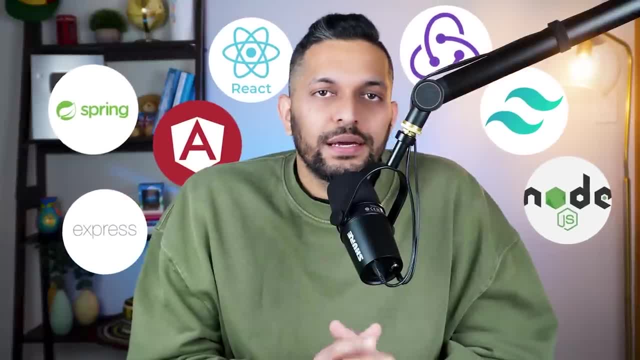 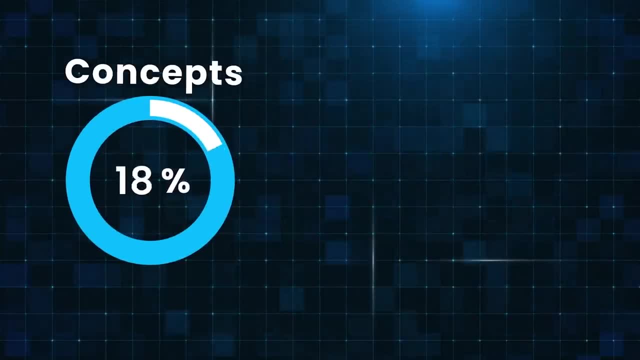 but the basics are just the starting point. There are a whole lot of other technologies that you need to learn in order to become an employable web developer, So I would not spend too much time here. I'll just learn the top 20% concepts that cover the 80% of use cases. 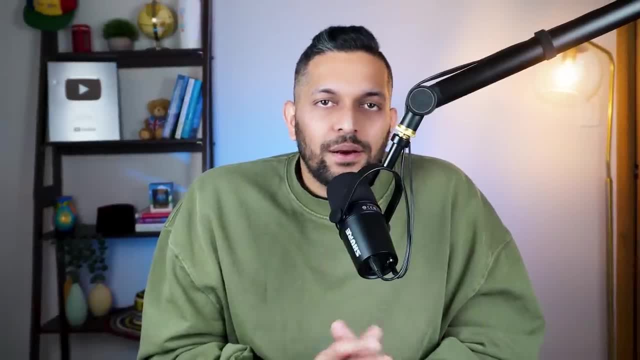 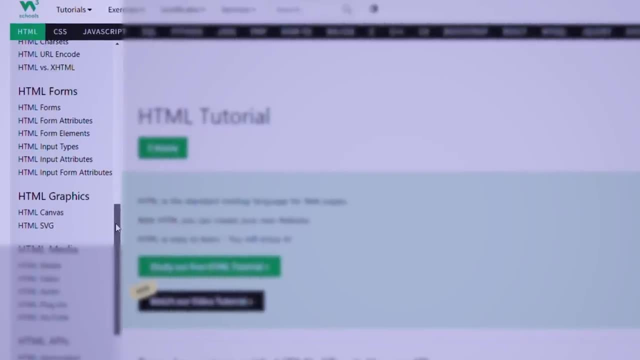 I'll learn the remaining concepts in the next steps To learn and test my knowledge at the same time, I'll go to W3Schools. For HTML, I'll start from the top and do everything until HTML Graphics. For CSS, I'll do everything until CSS Grid. For JavaScript, I'll cover everything until. 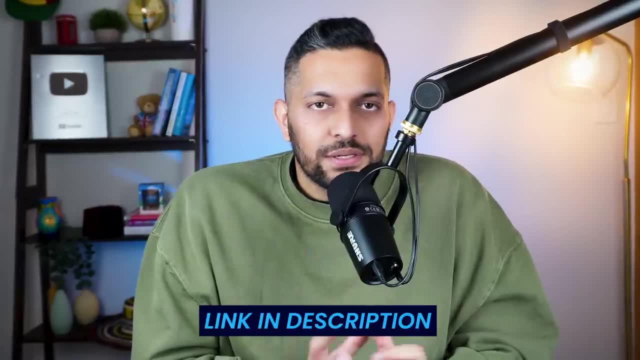 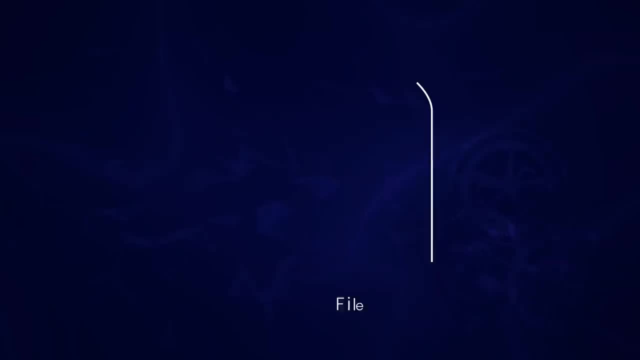 JSHTML DOM. I will add all the links to the resources in the description. Congratulations. you have covered 15% of what needs to be done to become an employable web developer, So let's keep going. When you start working with CSS, you'll see that same things repeat again. 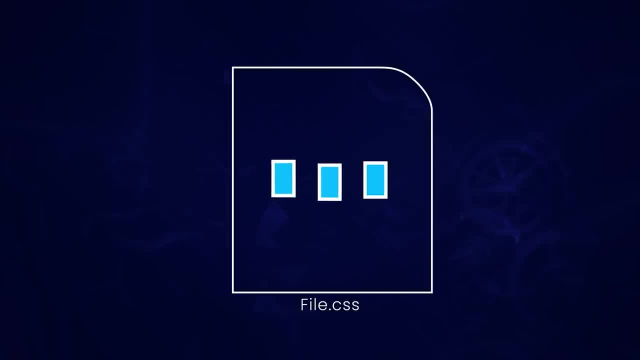 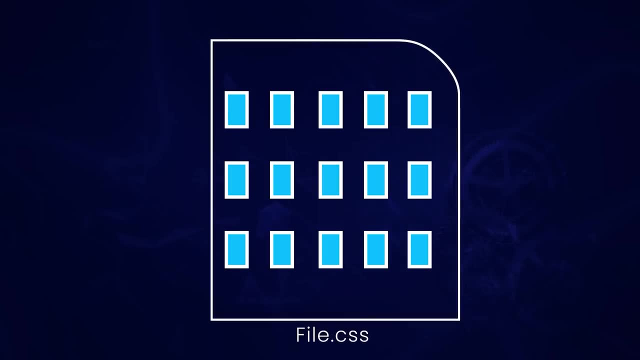 and again. You'll set height, add padding and fix alignment of different objects and so on, And when you do this for so many objects in your web app, your CSS files start becoming very big and hard to manage. On top of that, debugging becomes a huge pain because there is so much. 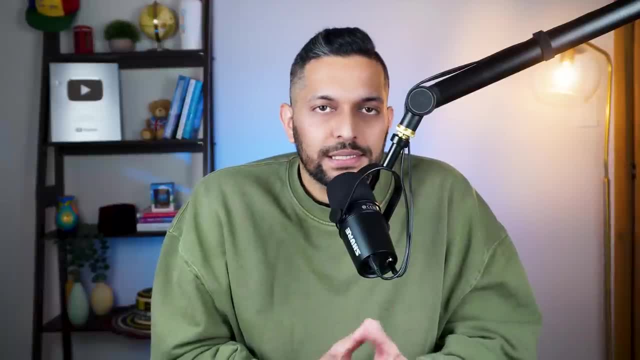 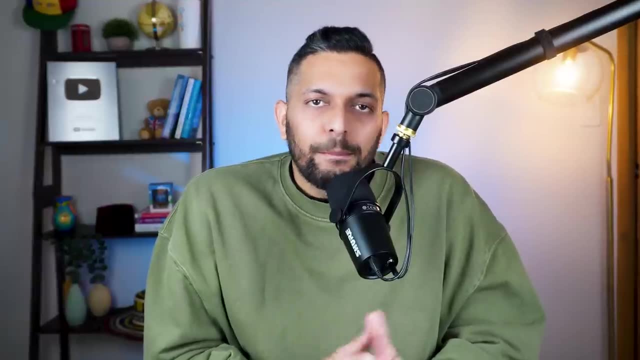 repeated code. To solve all these problems, you would want to learn a CSS framework. Now, there are so many different frameworks that you can choose from. Different people prefer different reasons. My reason is very straight forward. I would choose a framework that is: 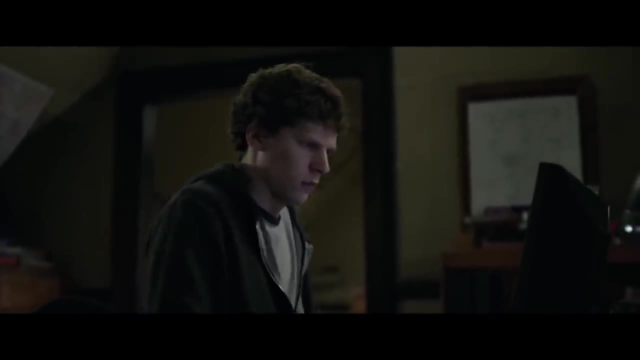 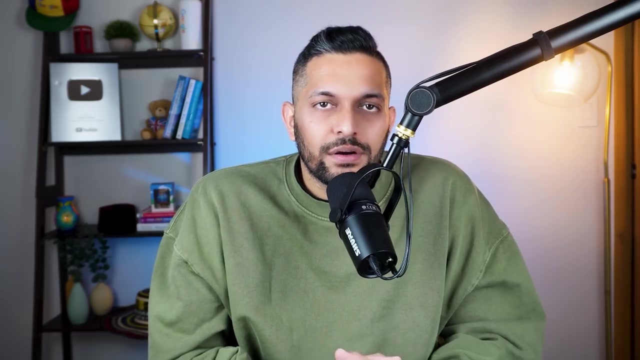 easiest to learn. Once I know the basics of CSS, I want to be productive as fast as possible. If you are someone like me, you would go for Tailwind CSS. Tailwind is a utility-first framework. In other words, Tailwind already has all the repeated code pre-written. You just need. 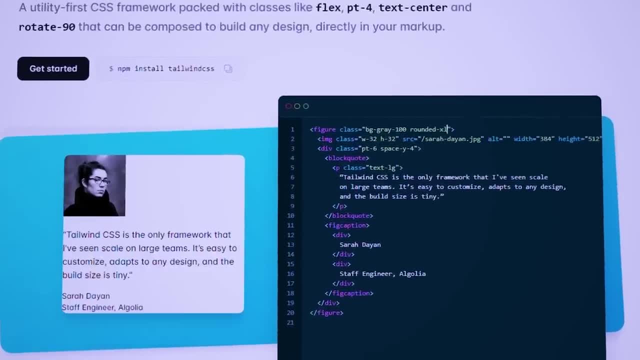 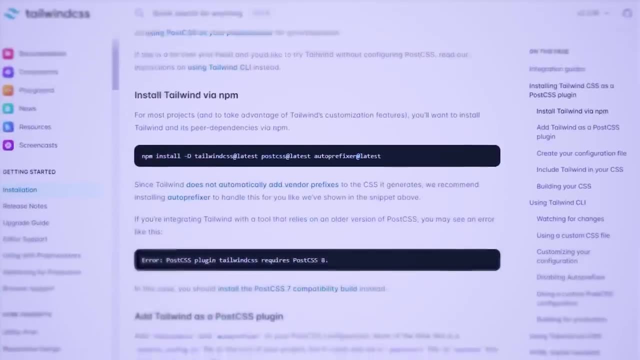 to go to your HTML elements and use it. This makes Tailwind very easy to pick for beginners. To learn Tailwind quickly, you can go to the Tailwind Playground and play around with the code. You can read their beautifully written documentation. You can also go to Tailwind Playground. 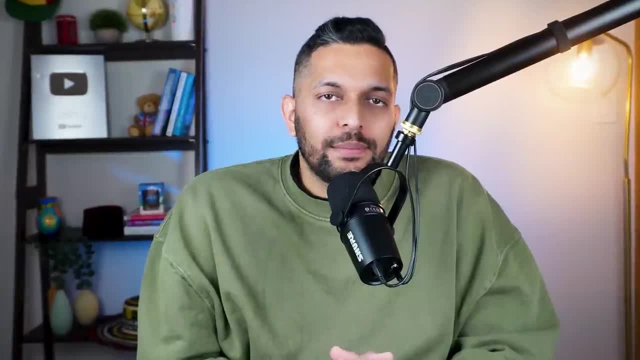 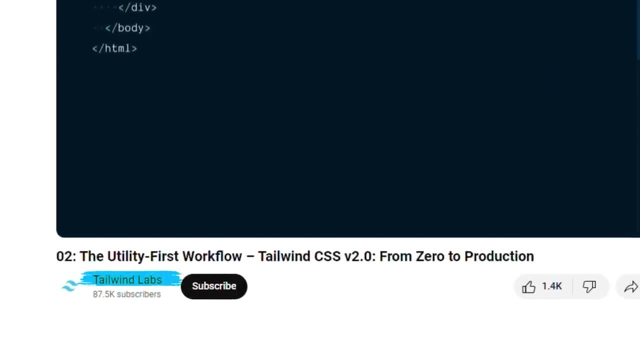 and test what you are learning in the Playground. If you already know HTML and CSS, this should be fairly straightforward. If you need more help, you can also check out the official YouTube channel of Tailwind Labs. We have covered another 5% with Tailwind. Let's move on to the 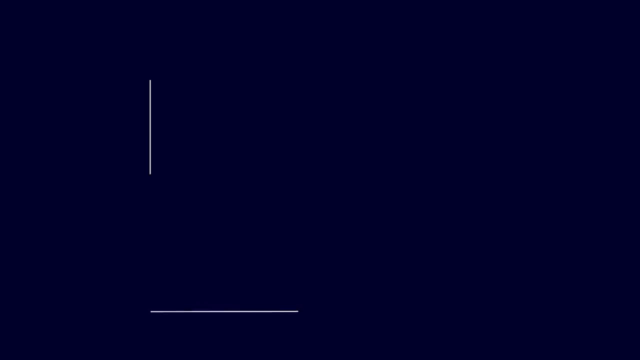 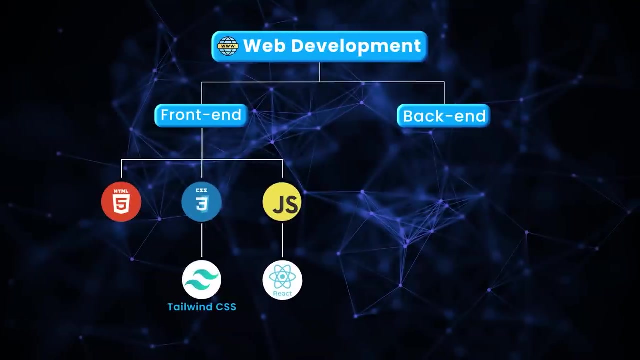 JavaScript framework. now, Just like CSS frameworks, we also have JavaScript frameworks to make our life easy. There are again many popular options here, But we will only talk about the most popular option, which is React. Technically, React is not a framework, It's a library. But that's not. 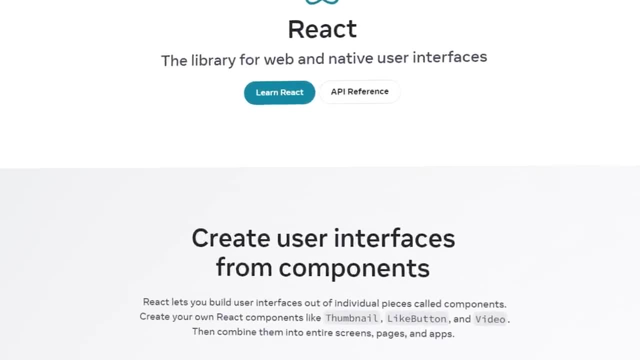 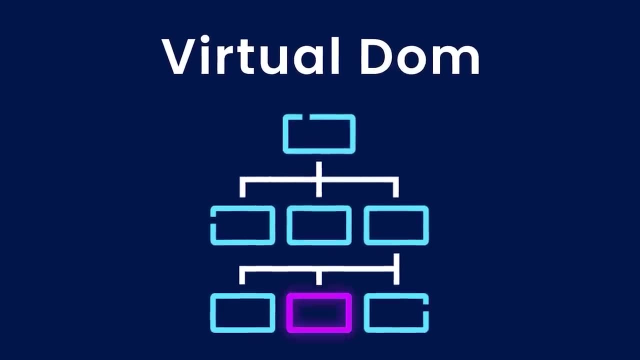 important for now. React makes building user interfaces more manageable by breaking them into small, reusable components. React has a virtual DOM that allows it to update only part of the webpage rather than re-rendering the entire thing. If you don't know what that means, don't worry about it. 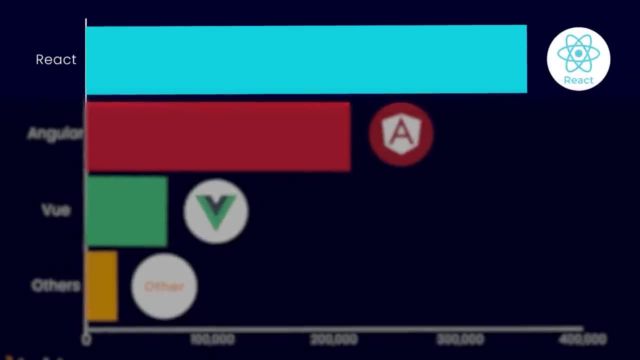 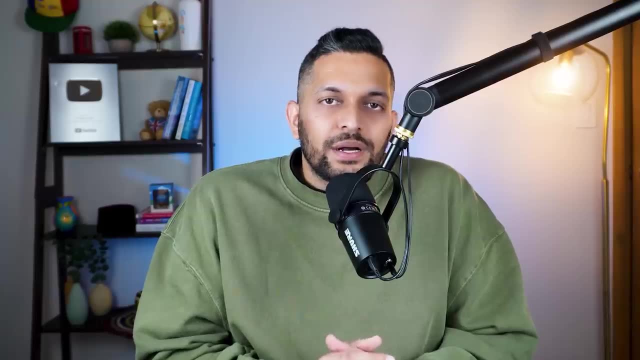 You will learn as you go. But why did I pick React over all these other options? My reason remains the same: I want you to get to a stage where you are building your own projects really fast, And React is among the easiest to learn and most in demand at the same time. So how do we learn React? 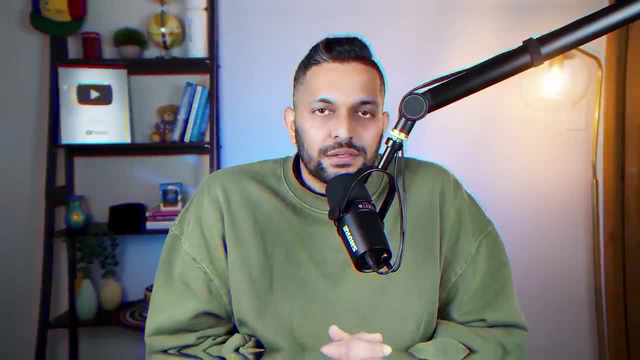 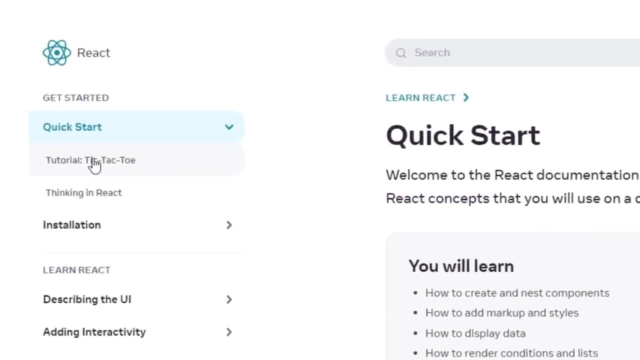 effectively. The official React documentation has made it very easy for us. They have a Quick Start guide which, according to them, covers 80% of the React concepts. This guide also contains a walkthrough of how to build tic-tac-toe in React, and they also teach you how to think in React. 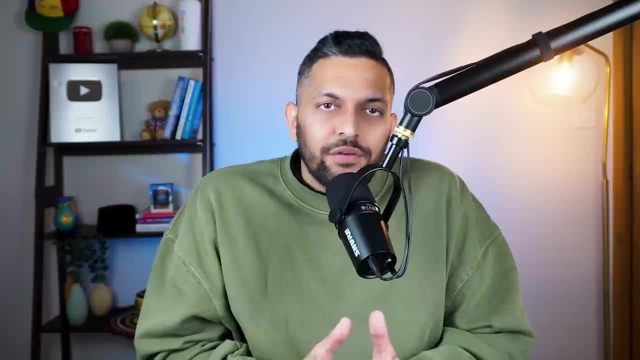 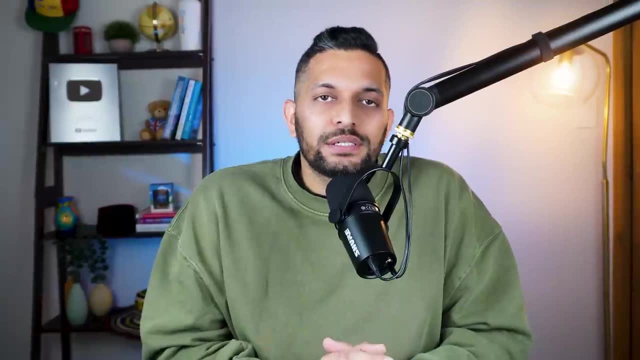 There is a Learn React section that I highly recommend you go through. But if you are short on time you can move on to the next step. With React basics you have covered another 10% So far. you have just learned the basics of a few technologies, But learning technologies and 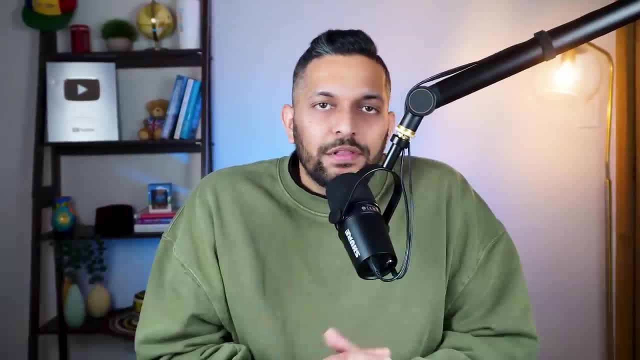 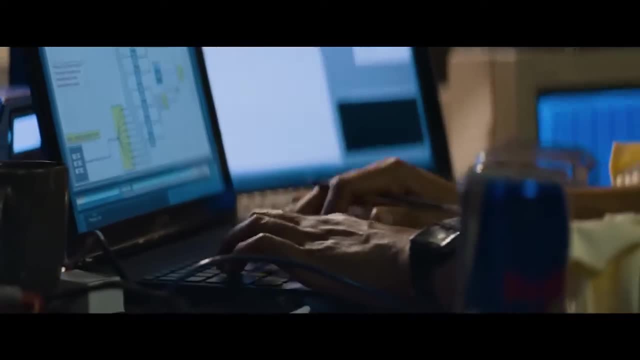 problems are two different things, And that's the gap we are going to bridge now With everything that you have learned so far. if I give you a new web app to build, most people are going to struggle with it, And that's totally fine. Struggle is where you actually learn, So if you are someone- 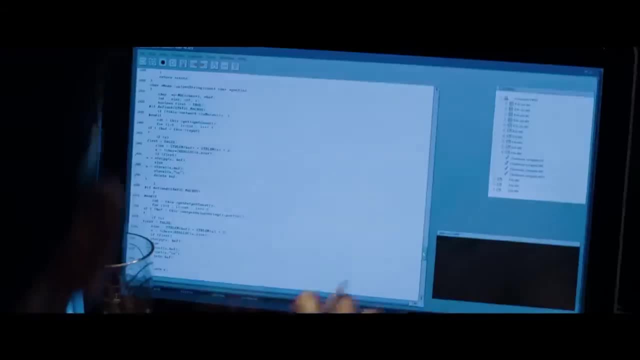 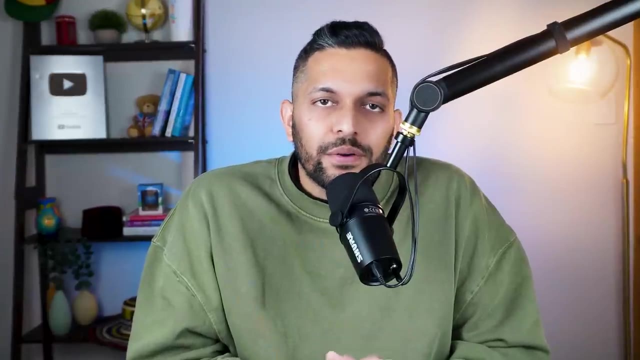 who enjoys the struggle. more power to you. Please go ahead and start building, because that's how you learn the most. But for others who need a little bit of hand holding in the beginning, I have a recommendation for you. You can start following along with someone who is building a real-world. 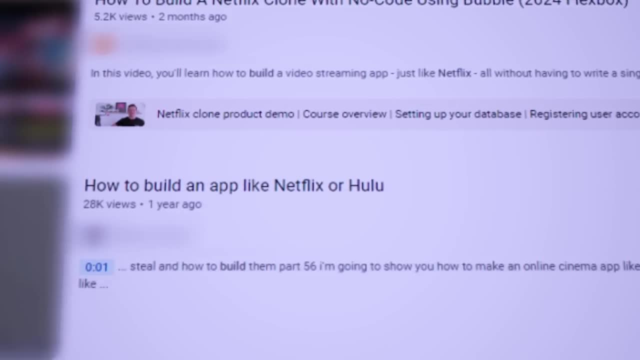 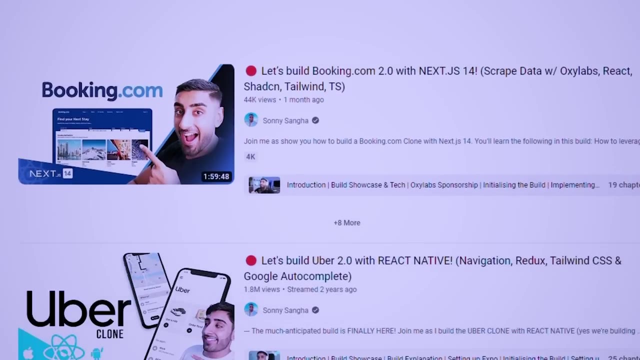 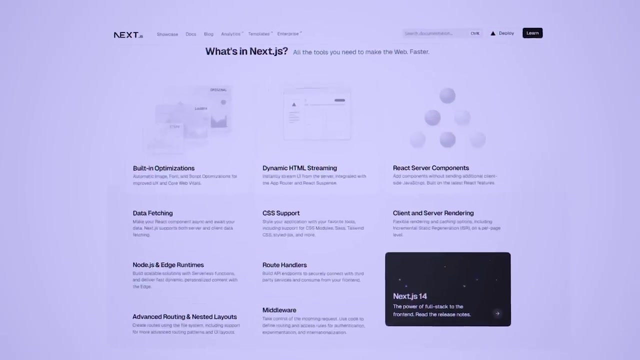 application. On YouTube you will find many people building clones of popular applications like Amazon or Netflix. My personal favorite is this channel by Sonny Sanga. His videos will introduce you to popular patterns in React. He also covers some new technologies like Nextjs. Nextjs is a React framework that enables extra features like server-side rendering. 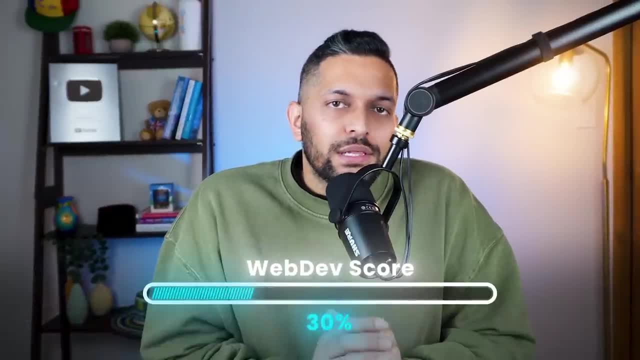 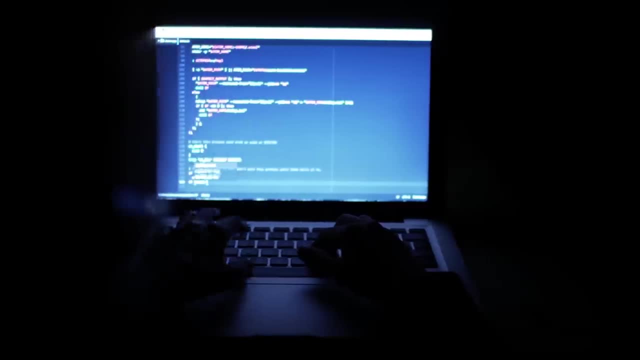 If you know, React Nextjs is very easy to pick. If you do all this, you will cover another 10% of your web development journey. Like I mentioned earlier, true learning will only happen if you start building new things by yourself. Building your own projects would be the 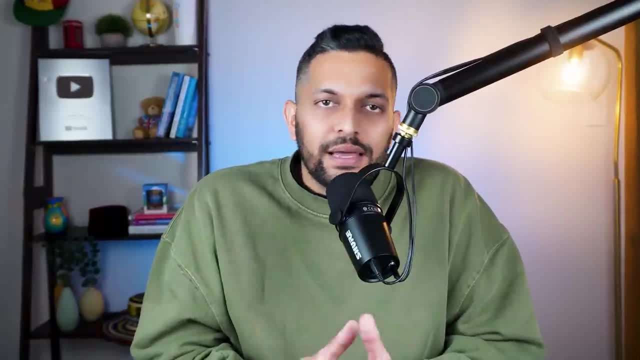 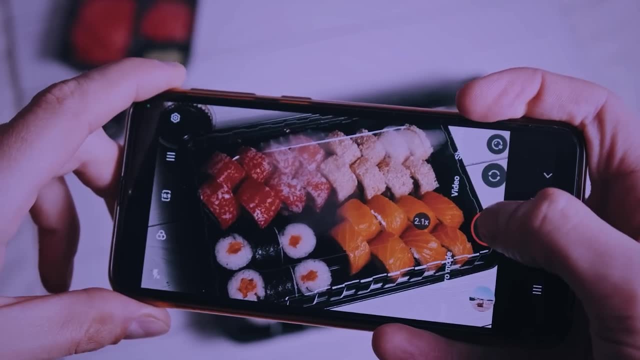 next 20% of your journey. But what should you actually build? I recommend that you build a basic version of Instagram app. Don't worry about videos or reels for now. Just build a version where people can share their photos and see a newsfeed containing pictures of their friends. You can also 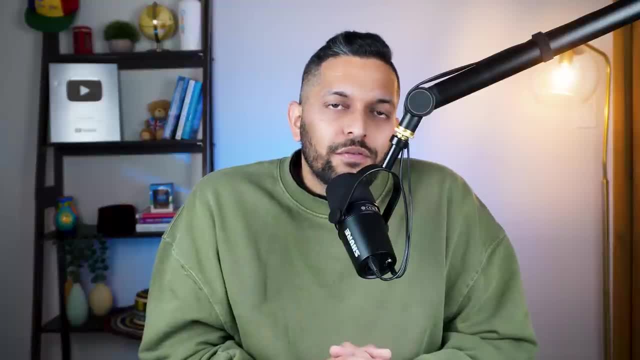 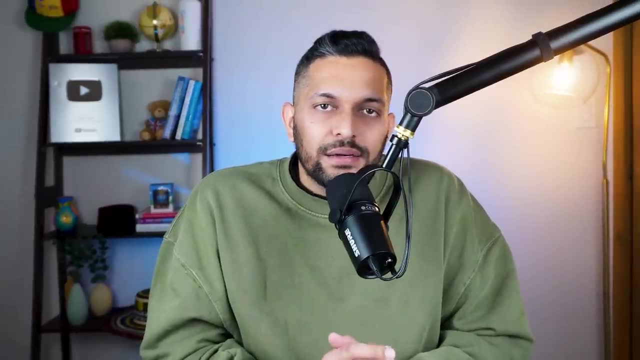 add functionality to like photos and add comments. Showing pictures from friends might not be possible right now because we have not covered backend yet. You can use some hard-coded URLs for now. After learning the backend, we will come back to this project and build the backend as well. 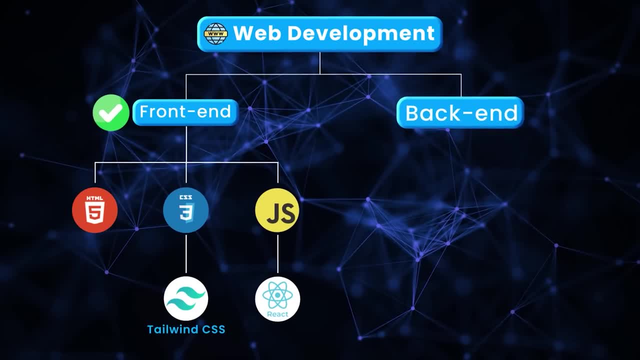 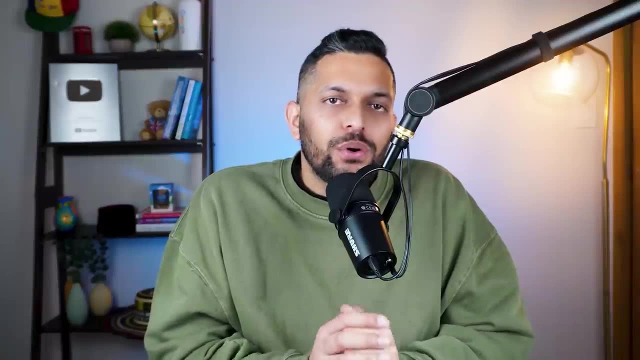 Now that we have completed the frontend part of the web development, it's time to move on to the backend. This is where people make their second biggest mistake, which is that they fall victim to the buzz around full-stack development. For those who don't know, full-stack developers work. 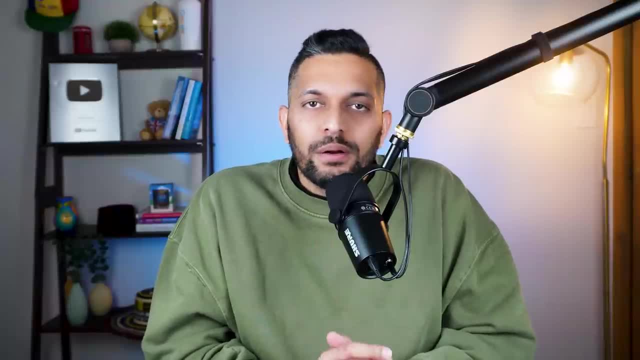 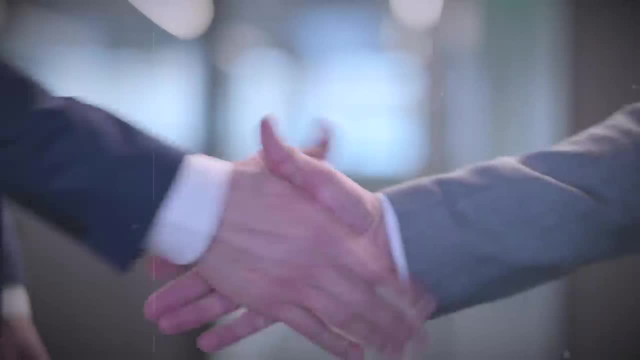 both on frontend as well as the backend. Now, I am not saying that you should not become a full-stack developer. Full-stack is a great end goal. The point I am trying to make is that you don't have to be a full-stack developer to find your first job. Frontend development is enough. There are many jobs for frontend developers, So I recommend that you don't rush into the backend development. Test yourself early in the job market to see where you stand, And you can continue learning backend on the side For the backend, we will again pick something that is. 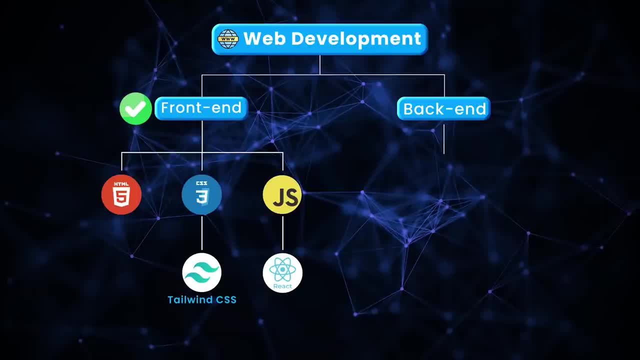 easy to learn. We already know JavaScript, So the easiest thing to do would be to use JavaScript in the backend as well. JavaScript was designed to be a scripting language for web browsers. To be able to run JavaScript on the server or backend, we need to use Nodejs. 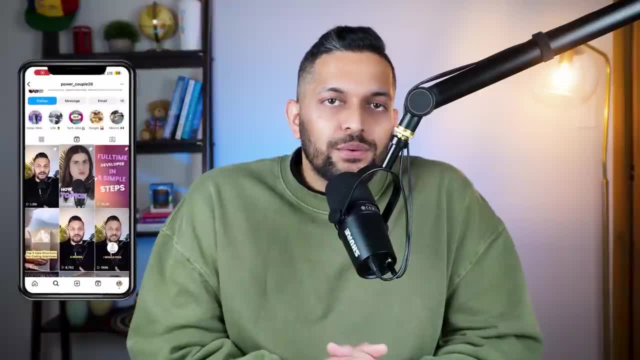 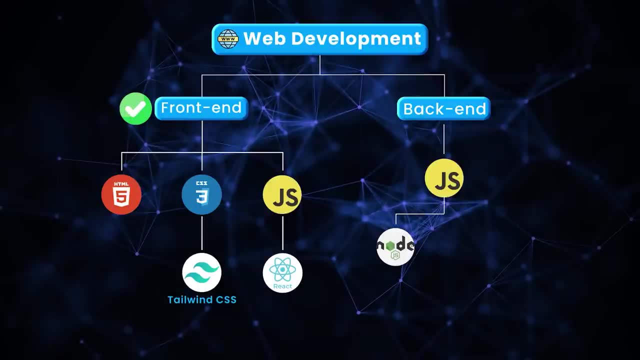 Nodejs is a JavaScript runtime for servers. If you don't understand what I am saying, that's completely fine. You will learn all this when you start working with Node. Now, similar to frontend, we need a JavaScript framework for the backend as well. 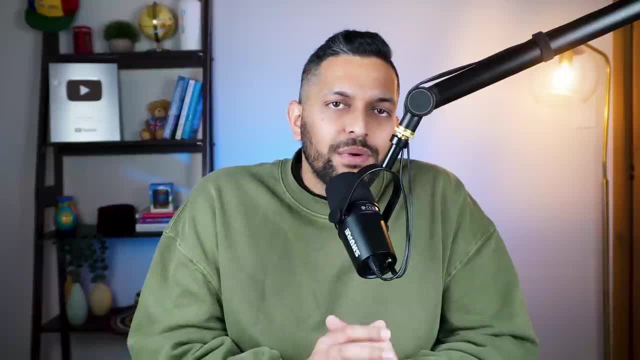 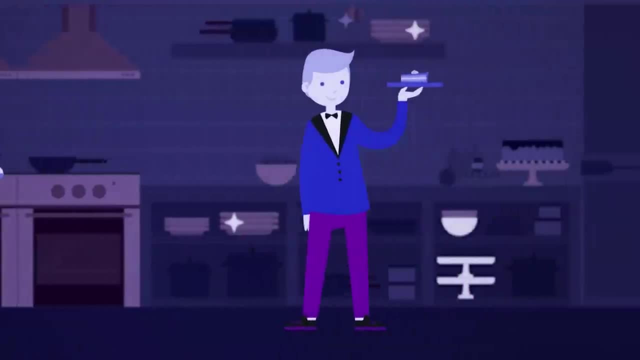 Express provides you all the tools you need to build APIs. Remember, in the beginning of the video we talked about how dining area is the frontend and the kitchen is the backend of a restaurant. An API would be the equivalent of the server of the restaurant, Basically. 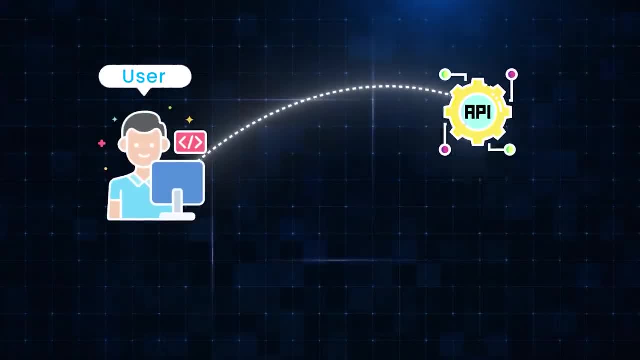 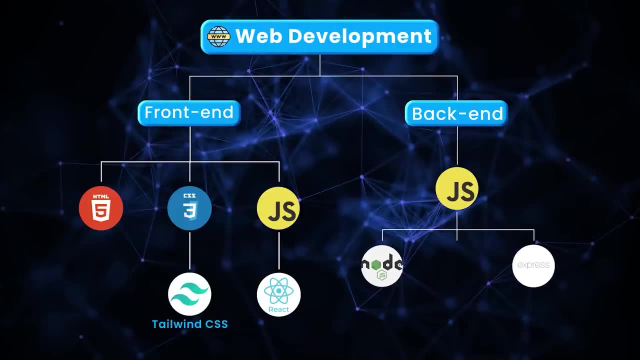 you place all your orders or requests with the API and the API responds to you with the information you need. An API does this with the help of the data stored in a database, So, in addition to Express, you will need to use a library like Mongoose to talk to the database. 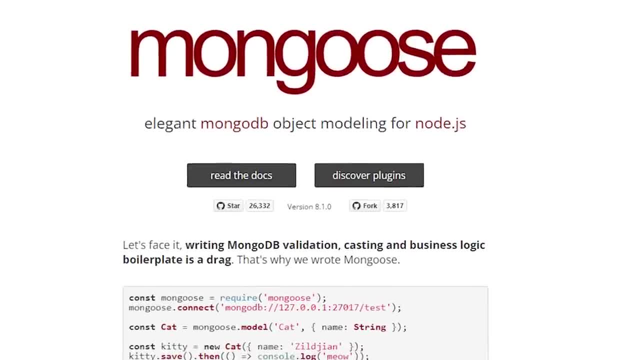 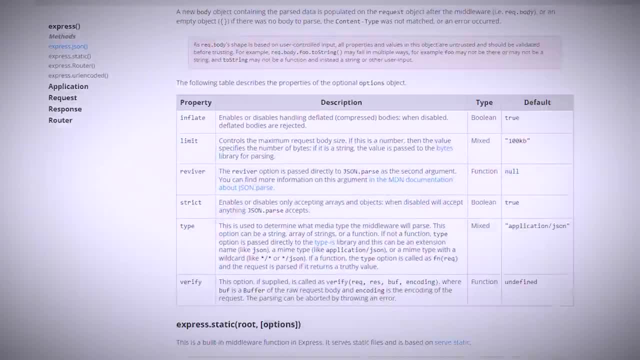 Mongoose is a Nodejs library for MongoDB, which is a popular database. I know all this sounds confusing, but it's not that hard when you start using it. To get acquainted with Express, you can quickly go through their documentation. But to actually learn Express and Mongoose- 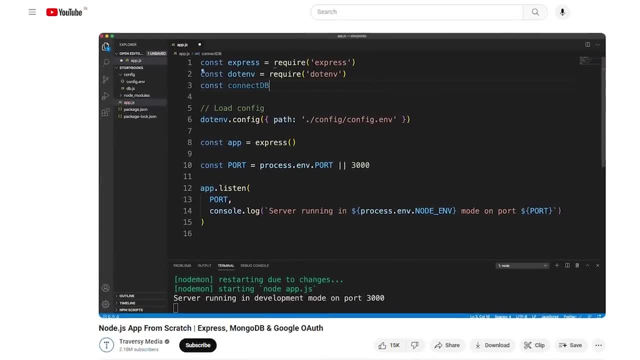 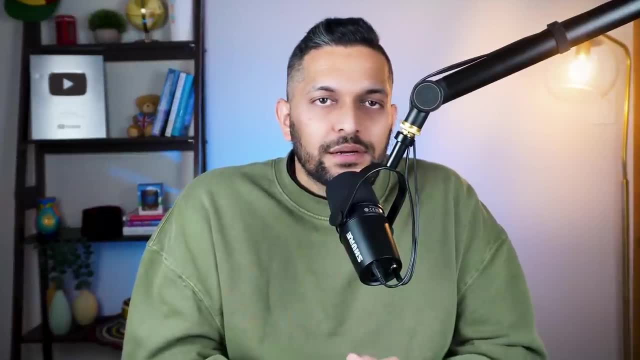 you can follow along with this video by traversing media and create a web app from scratch. I recommend directly by building, because if you have come so far, you already know enough programming to pick Express easily with this project And if you finish this step, you would have already covered another 20% of the journey. Now you are on the 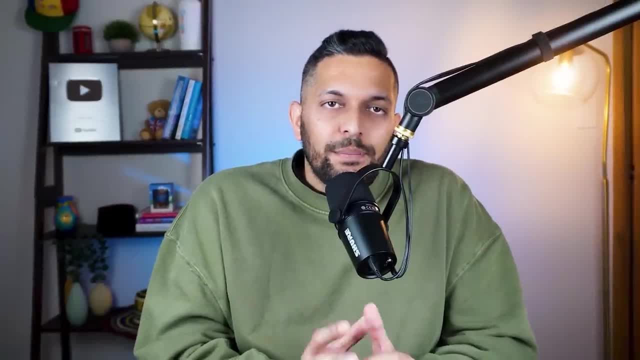 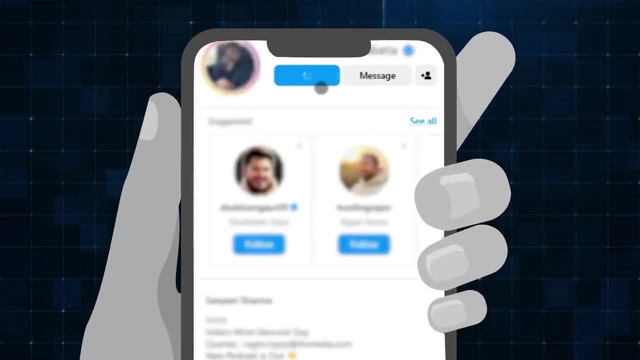 last leg. You need one final push, And that would come by building the backend of the Instagram project that you started. Add the capability to upload photos and follow each other by storing all the required information in a database. Create a newsfeed that contains actual photos. 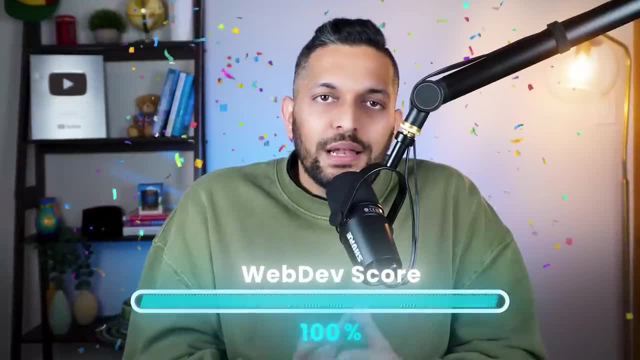 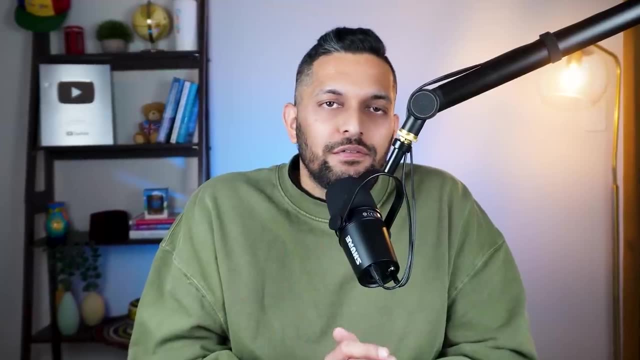 of your friend and not the dummy data. Once you do that, you will finish the last mile of the journey. And this brings me to the final big mistake many people make. They don't trust the process. They start this long journey of learning web development. They 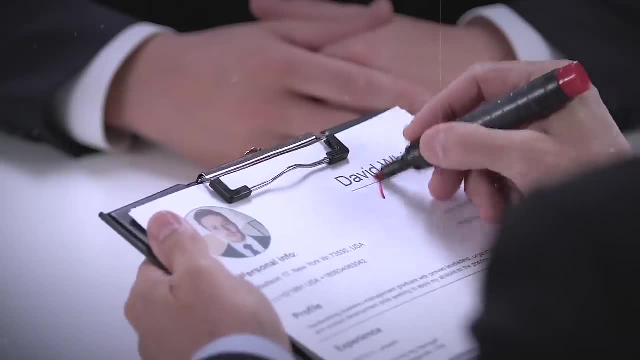 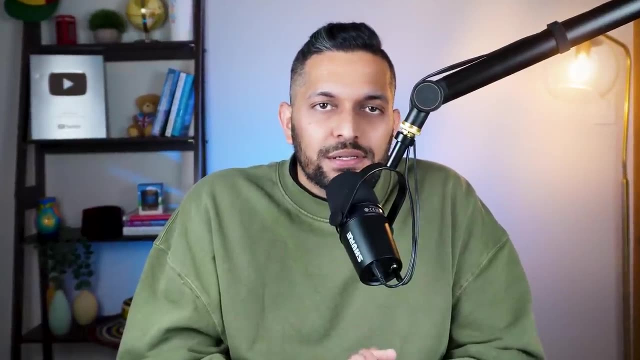 copy a few projects on the way and add them to their resume. Eventually, they are not able to find the job And they give up. Every step of the journey is important, So don't skip any step and trust the process. It might take you slightly longer, but you'll eventually get there. Now. 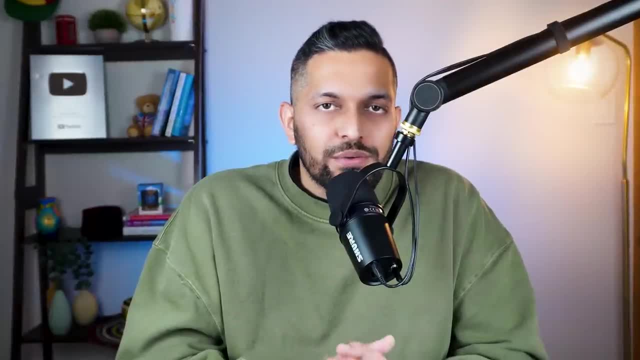 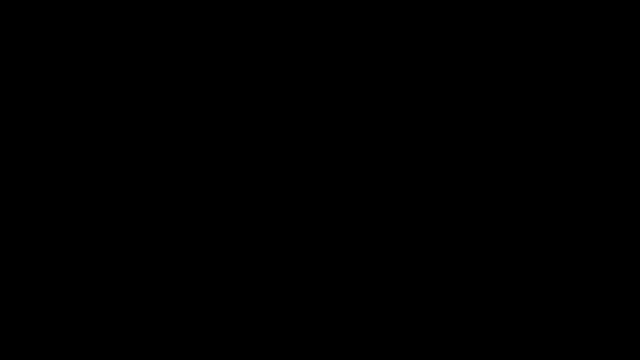 I did not get a chance to cover how to prepare for coding interviews in this video. If you are interested, you can watch this video. My name is Sahil and I'll see you in the next one.